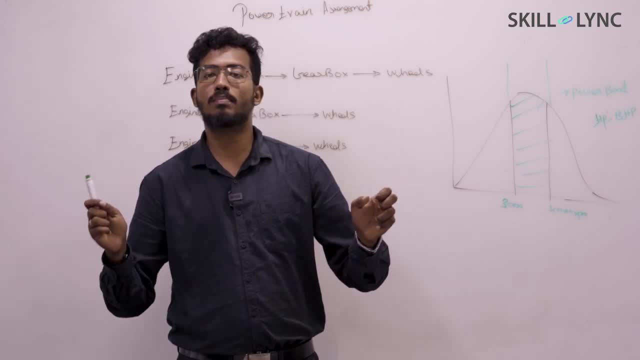 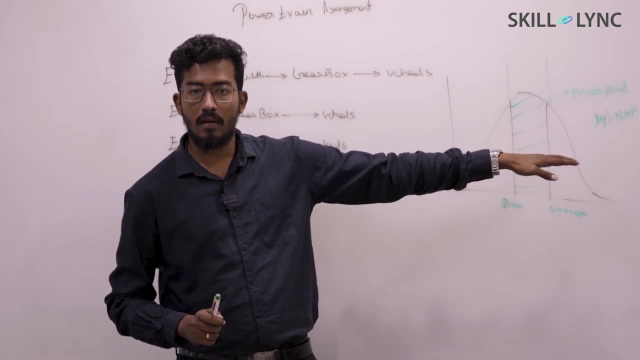 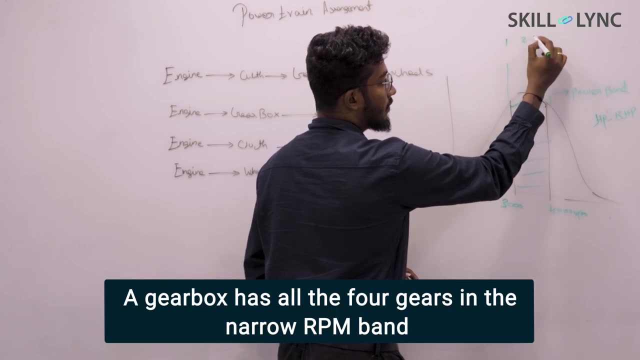 of your final gear, you will be able to experience the fullest power from the engine. this is the biggest drawback. to hide this drawback of engine, the setup gearbox, how we are going to do it. they're going to have all the four gears in the power band right. so it's kind of you know you look. 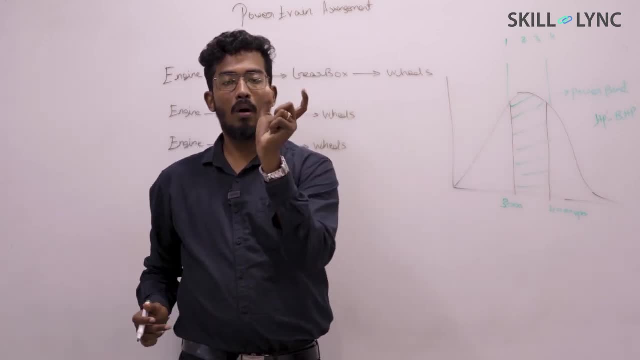 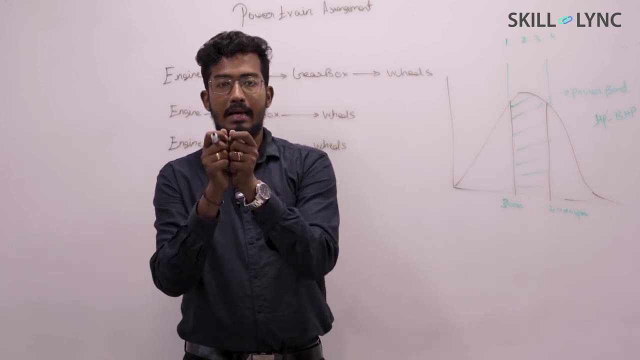 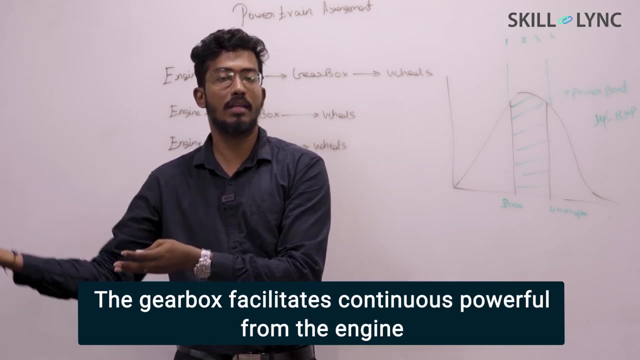 at it. it's very narrow right. so we're going to have all the gears correct: four gears, five gears in the respective power band, which will elongate the power band and make it seem like continuous process, continuous power flowing from the engine right, which is actually not right. so that's why. 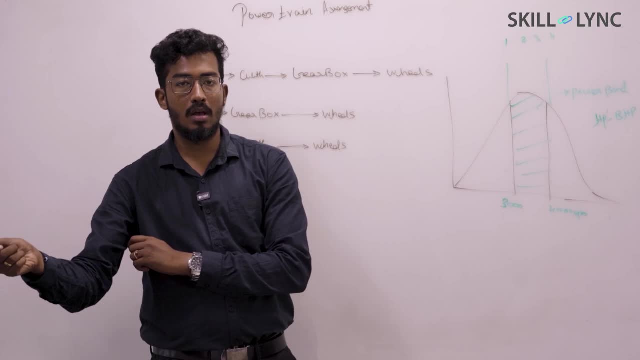 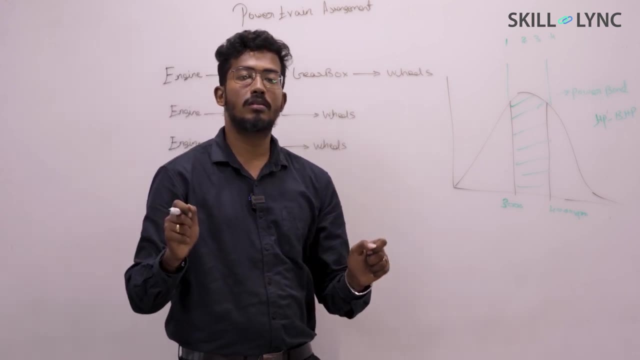 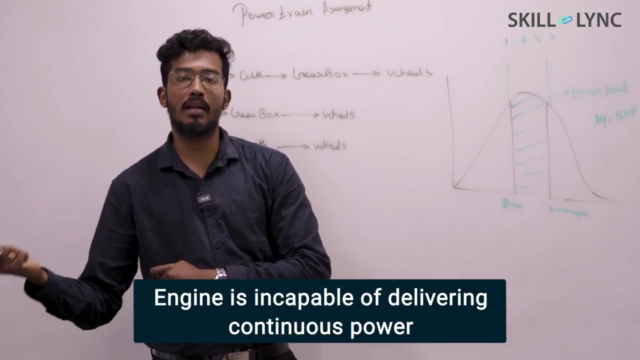 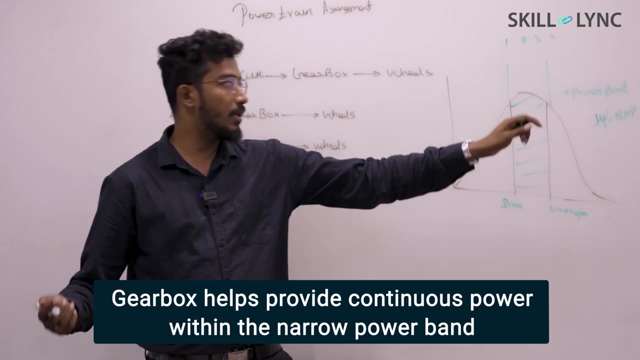 gearbox is hiding the disadvantage of an engine and showing as if engine is capable of providing a continuous power. right, and that's also the reason why gearbox cost is pretty much higher than the engine cost, because engine is incapable of delivering continuous power. then gearbox kicks in and make the discontinuous power into continuous power at the power band level right. so 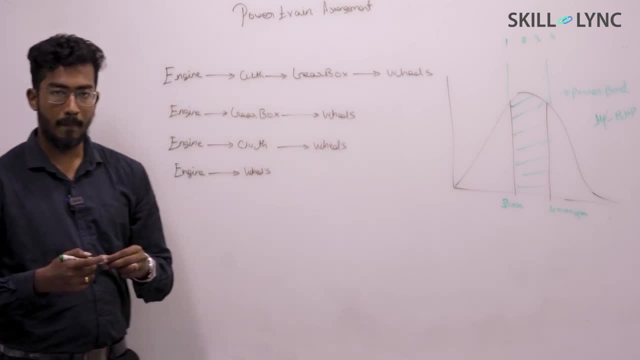 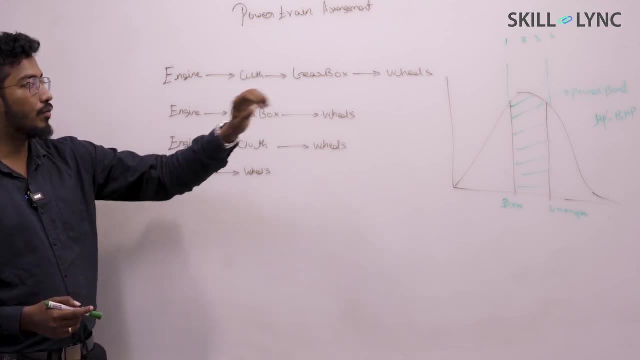 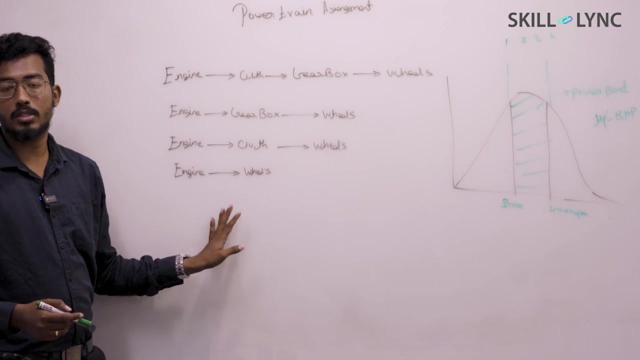 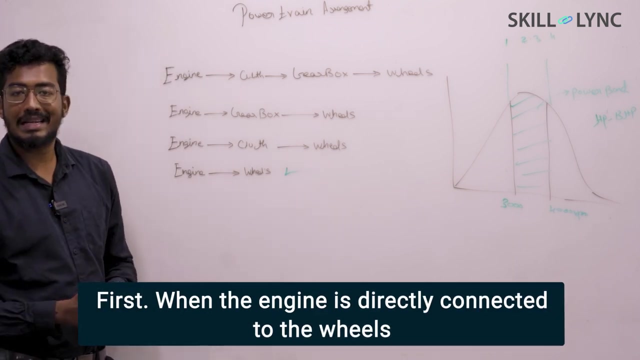 in addition to that, we're going to look into four different arrangements of a powertrain, right? so we're gonna go start from the convention all the way, narrow down to what's possible, what's practically possible and what's not right. we'll start off with first. engine directly connected to wheels is practically impossible. 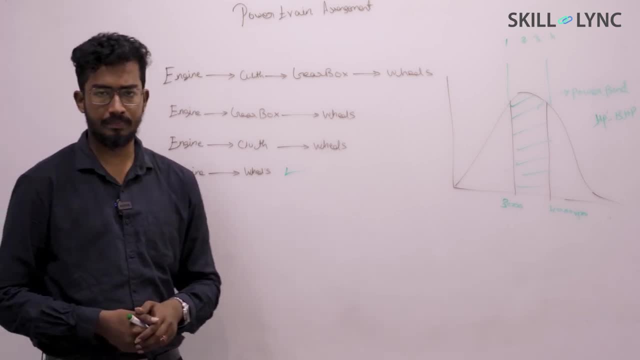 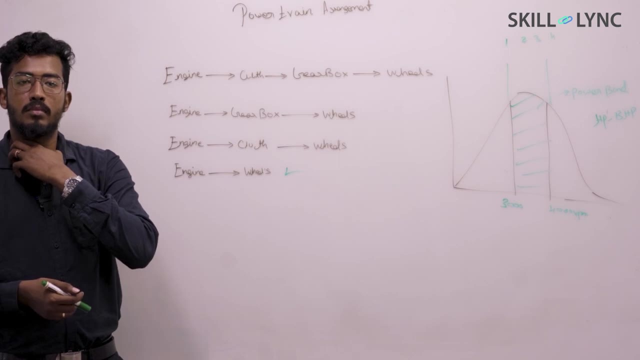 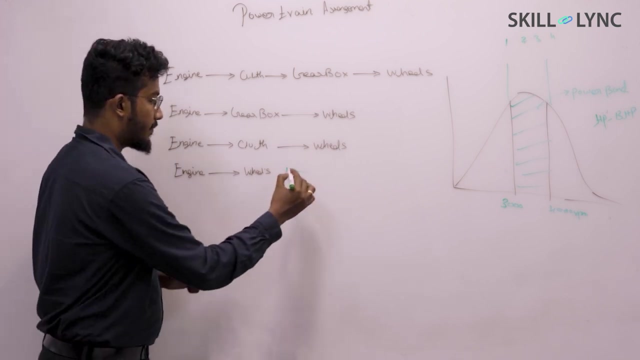 think about it. you're just directly connecting the engine to wheels. try to drive off. what would you experience, right? you will experience a direct connection from the engine to beat, which is not good. you want a disconnecting member, right? so this is not going to work right. and the tricky part is: 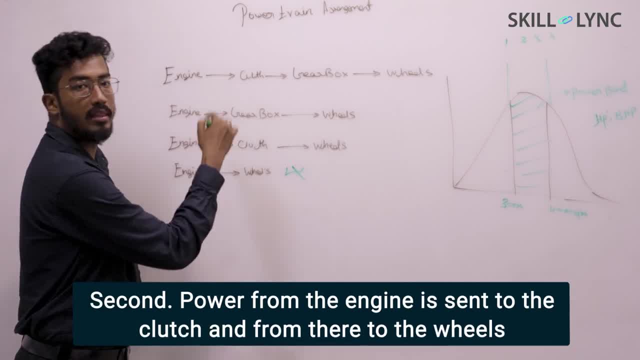 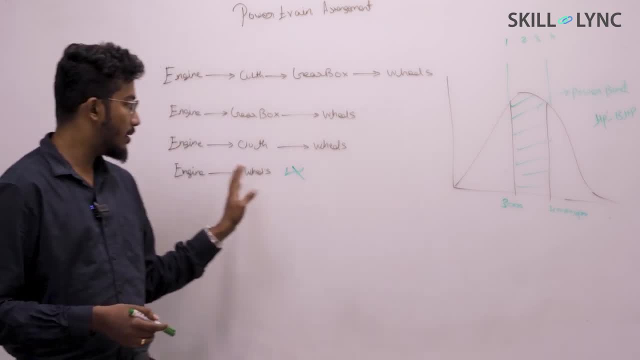 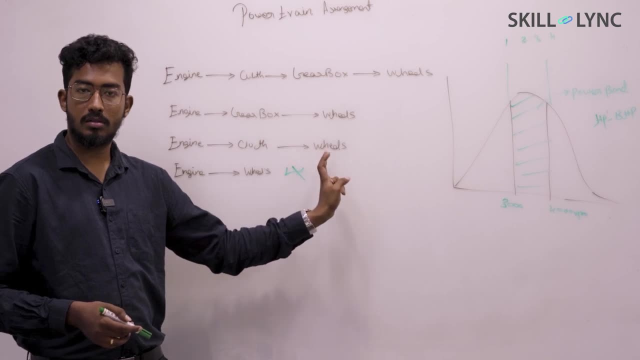 engine power is going directly to the clutch and the wheels. just try to think about it how this could be done. you have an engine- power is coming from the engine- and then a clutch built into the chocolate trás. the wheels willfeed. like this: the power is coming from the engine. now you don't have a gearbox. you 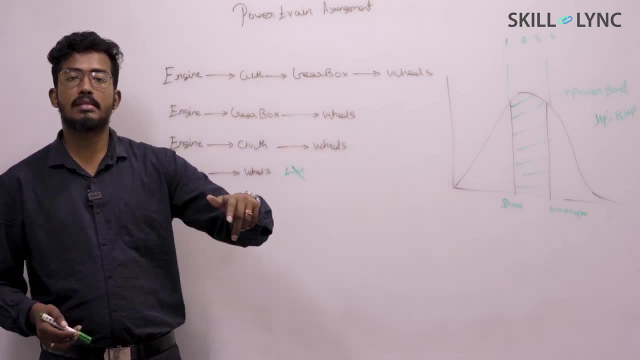 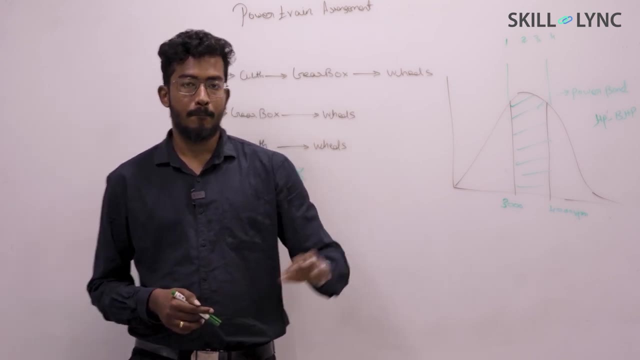 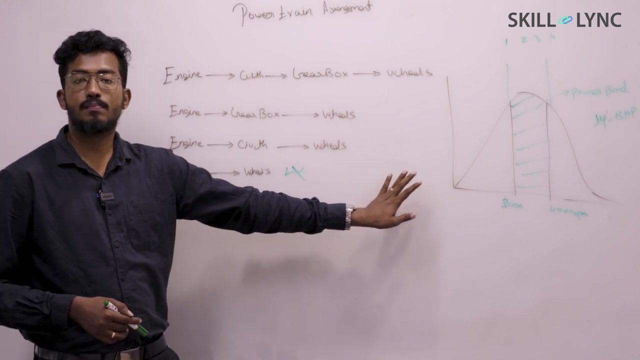 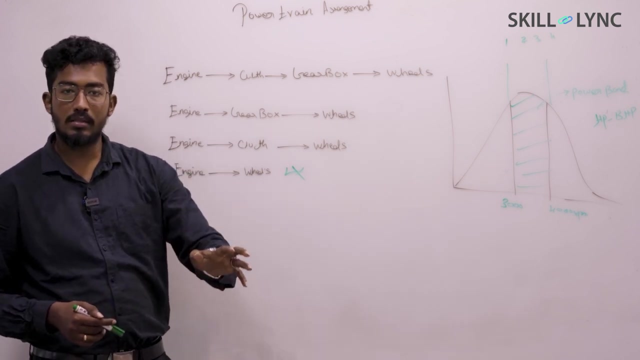 don't have a gearbox, you have only clutch and from there you're directly corresponding to the wheels. what would happen if you replace your existing setup to this setup in your wagon? just think about it now. vehicle is daily. this is mostly used in a daily, on day-to-day basis, such as your scooties, mopeds. 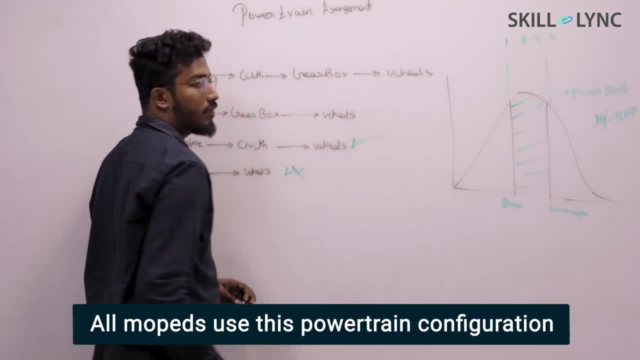 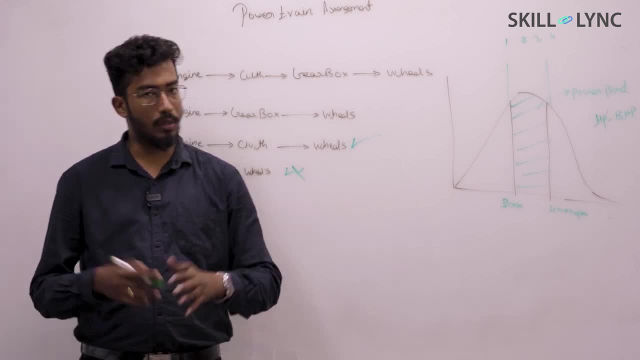 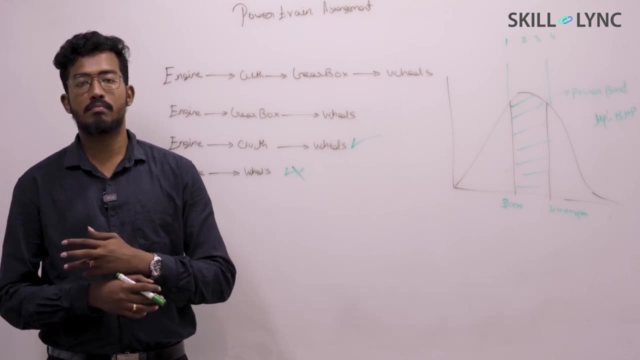 they use this method of power train configuration, you might have wondered how they're even doing it right. is it automatic transmission or is it a cvt? no, the very simple answer to it that's centrifugal clutches. all these scooties, mopeds, they use centrifugal clutch to transmit the 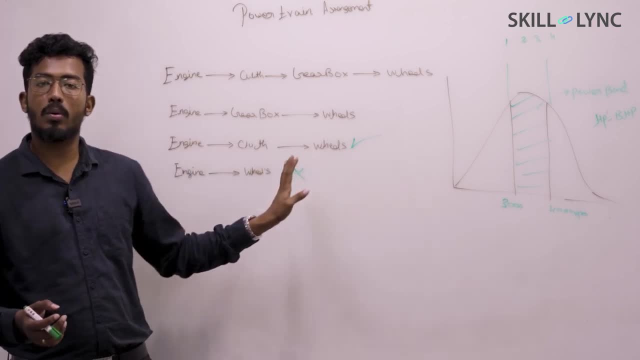 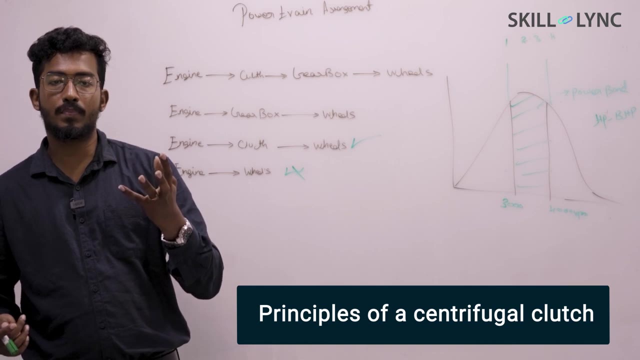 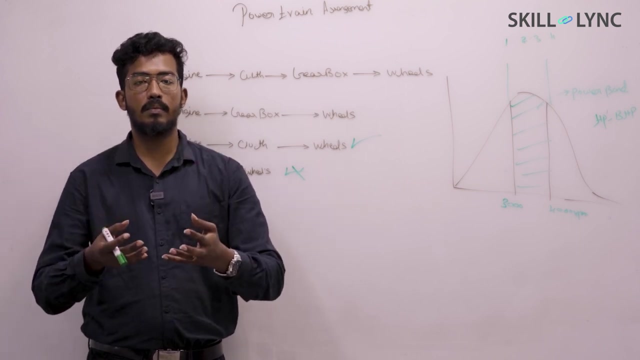 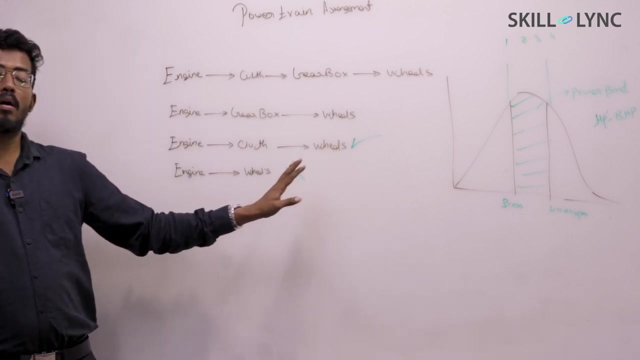 engine output directly to the wheels without needing any gearbox in it. how is they going to do it? a centrifugal clutch works on a principle of whenever you you stay in idling rpm, it doesn't get contact with the outer rpm or or the wheels side right. so if you run beyond 1000 rpm or you rev the vehicle beyond 1000 rpm, 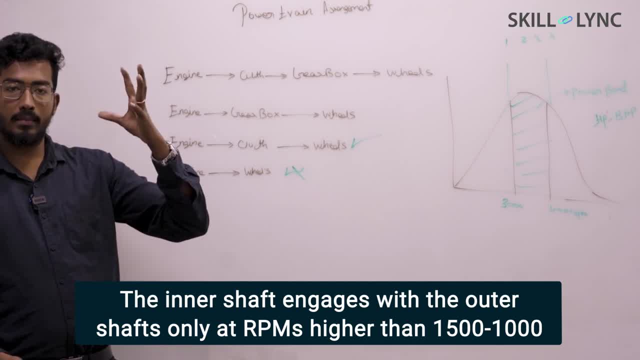 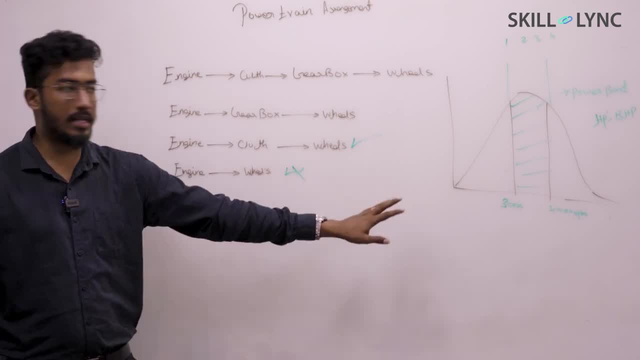 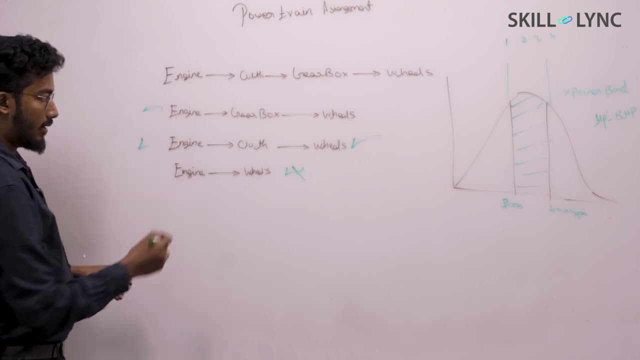 say you are under 1500 rpm, now you're expanding it. it starts getting contact to the outer surface. hence it will transmit the power from the engine to the wheels. that's mostly used automotive transmission in the third category. second, again, think about it. this time we are. 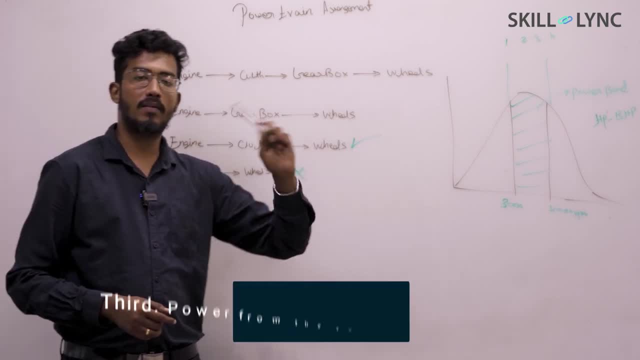 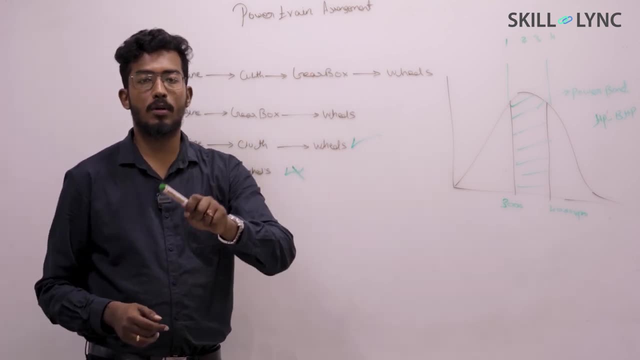 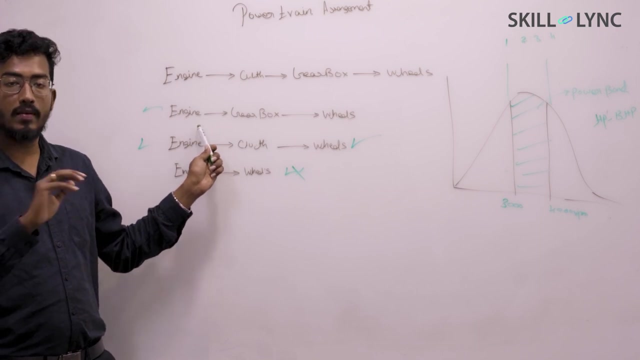 eliminating clutch with the design I talked earlier- engine- the power is directly going to gearbox, and then it's been converted to the wheels. right, take a pause, think about it. it's even possible to make a product with this design too. you don't have a clutch now. you don't have a clutch. 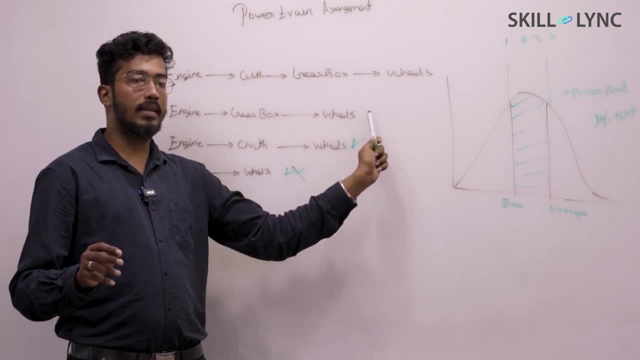 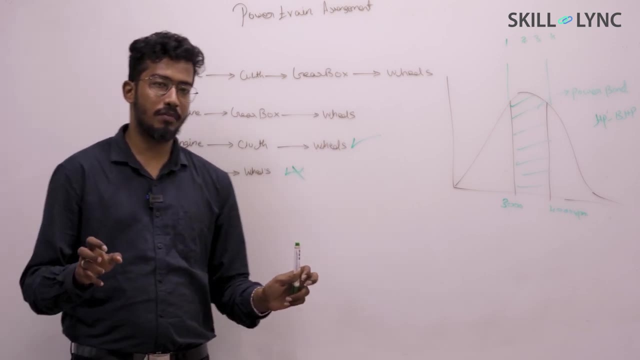 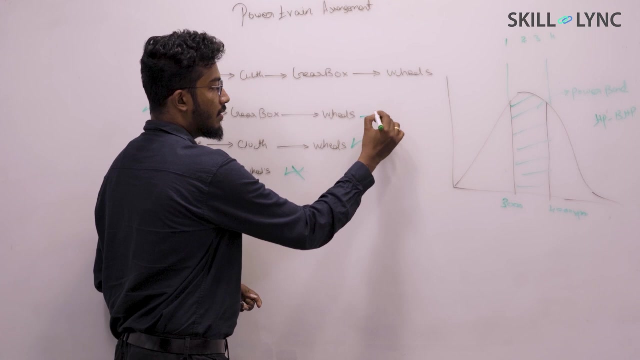 engine power is directly given to gearbox and followed by that, it's going for the wheels. yes, it's possible. there's only one product in this category, I think, which most of you might have not about. that's TVS drive right, that's the only one product which works on class 2.